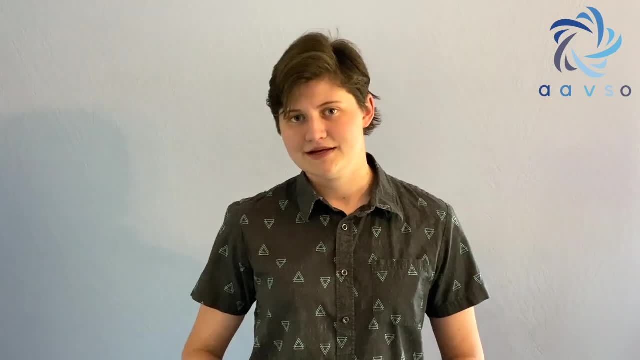 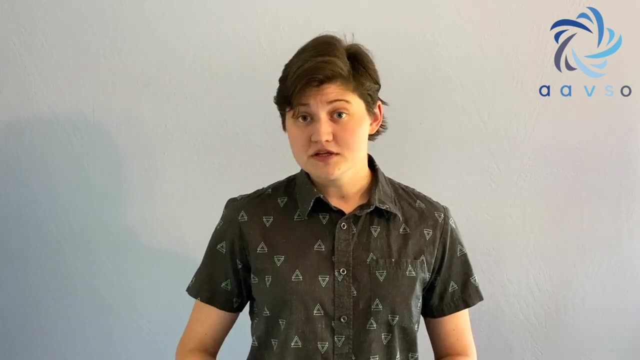 at first, but the lower a star's magnitude, the brighter it is. There are many resources available online at AAVSOorg that can teach you how to look at variable stars with a small telescope, binoculars or even your naked eye, And even though light pollution is annoying, you can still take. 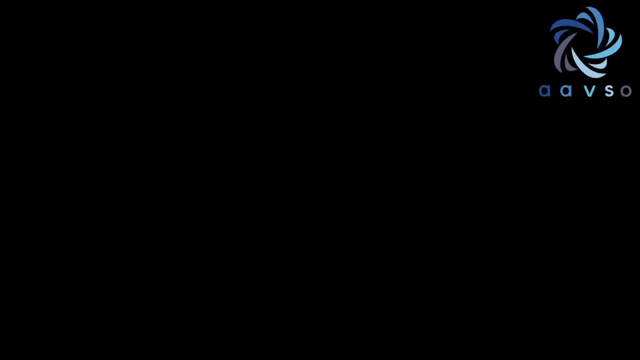 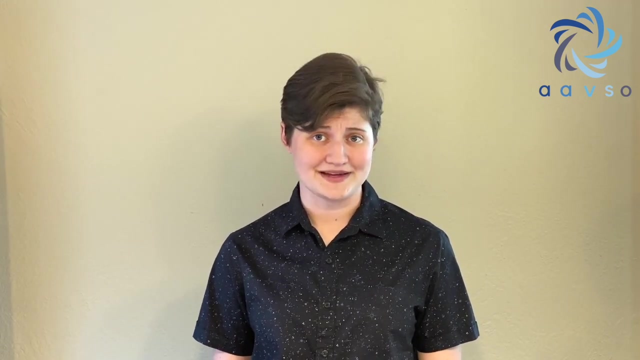 photometric and spectroscopic data inside city limits. We can't always get out to the country where the stars are the best, so it's good to know that we can still observe from home. Next we have Lauren talking about stellar spectroscopy. 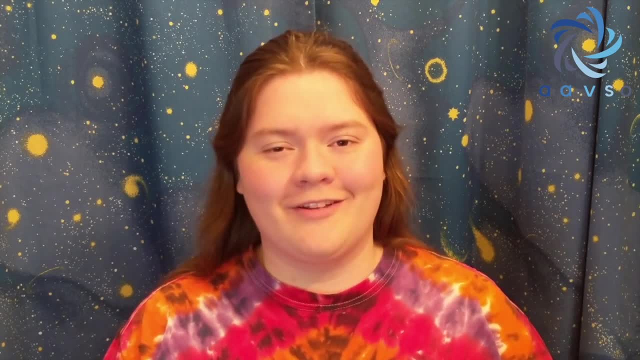 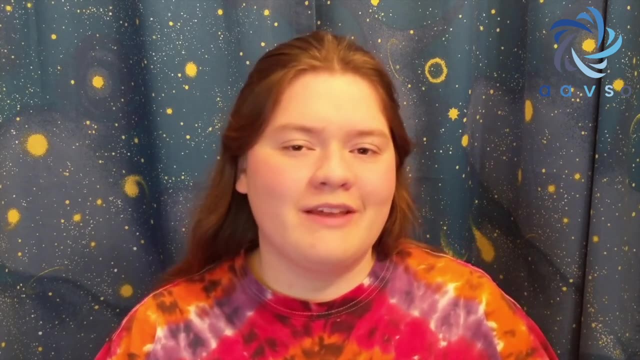 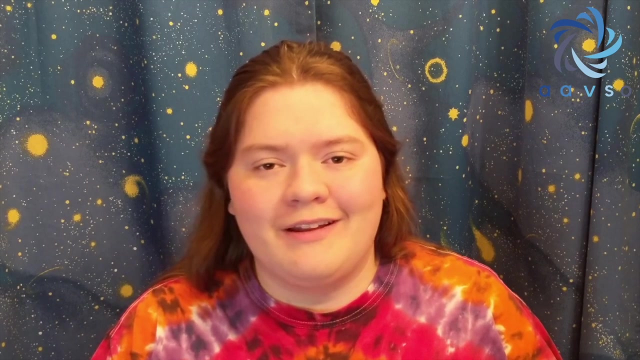 My name is Lauren Herrington and I'm in love with the stars. Given that fact, it's a wonder I didn't join the AAVSO sooner. The thing is, when you think about the AAVSO, you're probably thinking of making magnitude estimates or doing photometry, In other words. 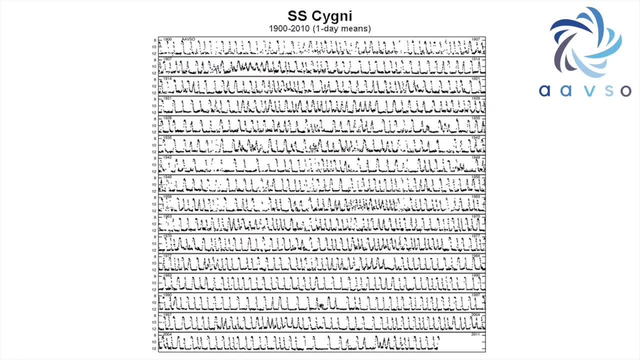 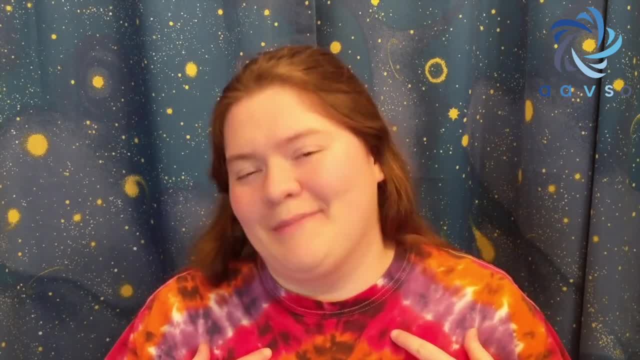 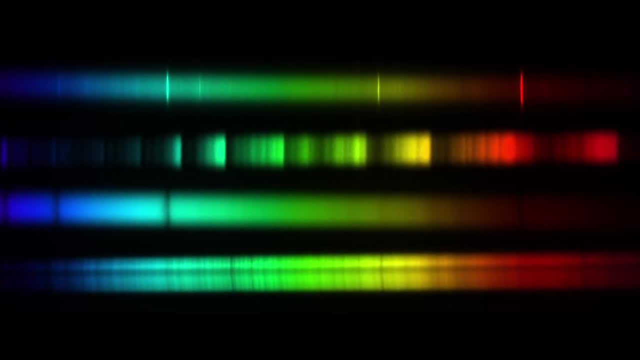 watching how the brightness of a star changes with time. Now, there is a lot we can learn about a star through its brightness, but me, I'm all about color: Astronomical spectroscopy. You see, spectroscopy is a way to learn not just how bright a star is, but which atoms. 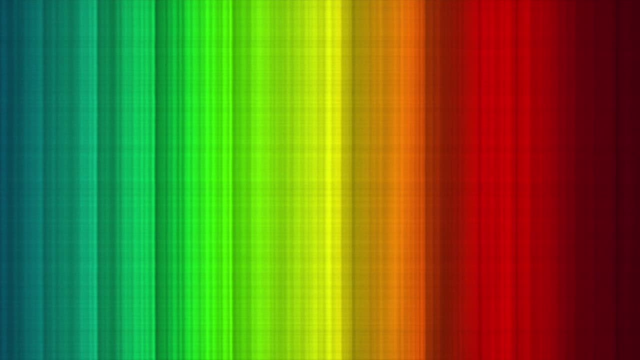 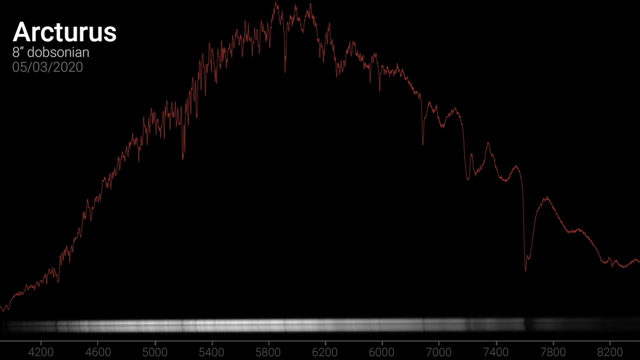 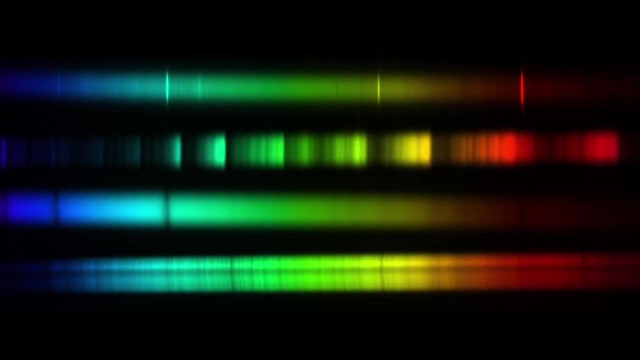 and molecules are buzzing around there in the strange physics of its photosphere. With spectra, you can measure the temperature of a star without needing to use a thermometer. You can measure the pressure on its surface without a barometer. It's an exaggeration to say that spectra are how we know most of what we know about the universe. 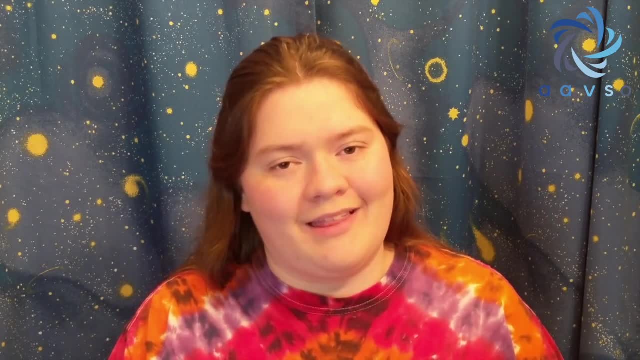 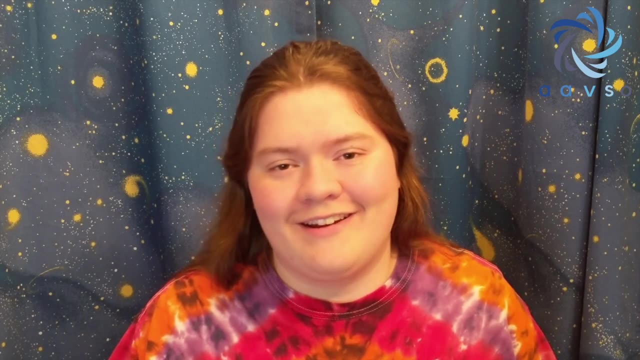 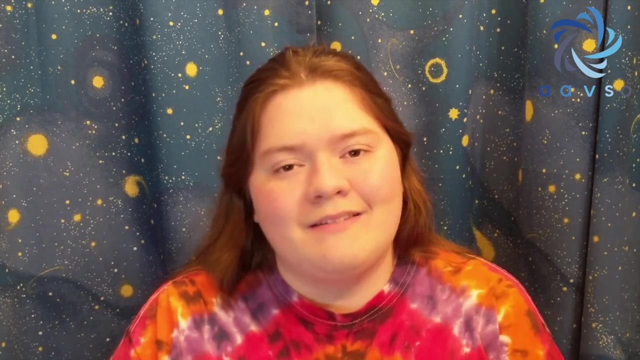 For years I admired spectroscopy from a distance because I was just certain that it would be too expensive for me to try for myself. I mean, I'm just a student on a budget. I can't exactly afford some big spectrograph or beefy tracking mount. But then I started experimenting. 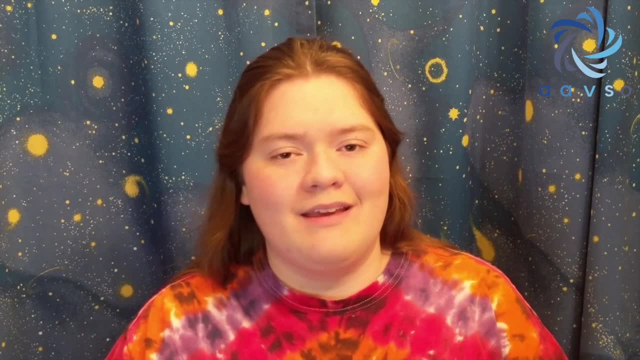 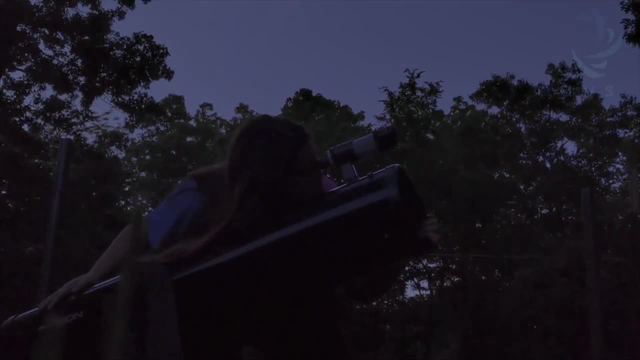 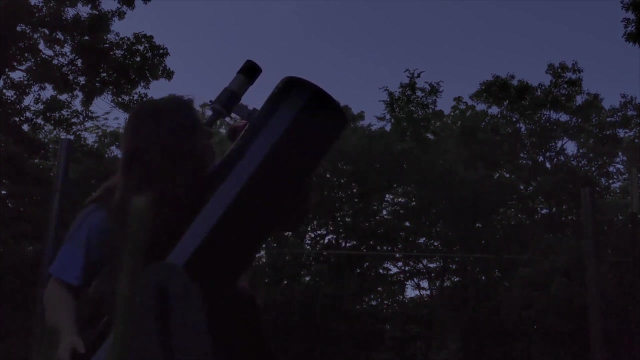 It turns out, all you really need to do. spectroscopy is just a camera, a diffraction grating and a small backyard telescope. Now I'm out under the stars every night, shooting spectra using the very same telescopes I've been using for visual observing for years. 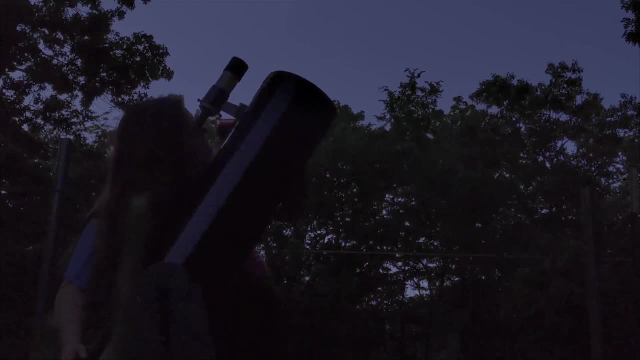 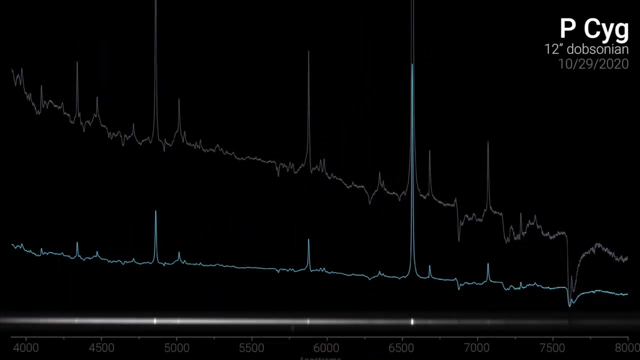 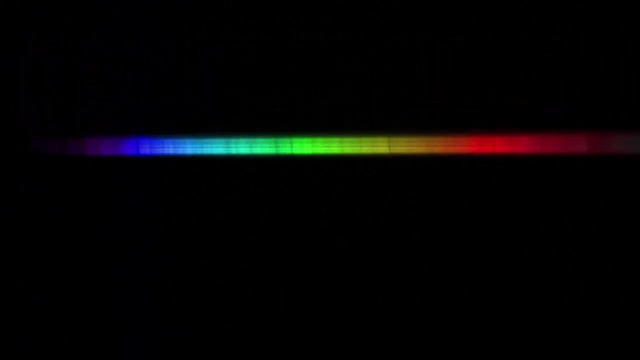 With this simple equipment, I've seen fantastic things: Hydrogen emission in the thin outer atmosphere of a giant star, Blue shift in a dying star's stellar wind, Even a fine forest of metallic spectral lines that betrayed the signature of a star, just like 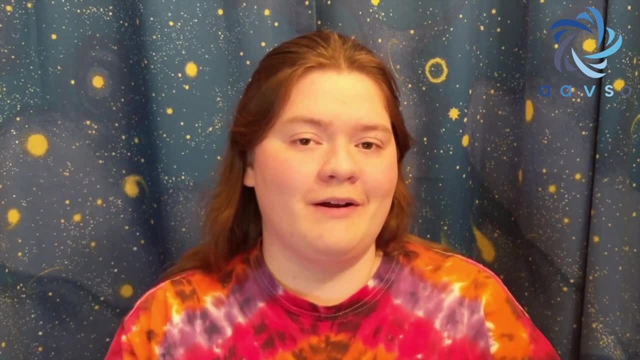 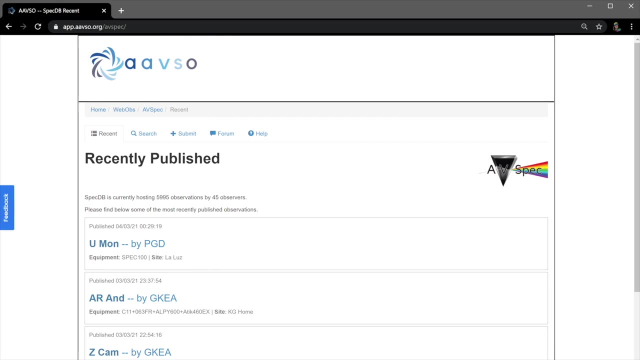 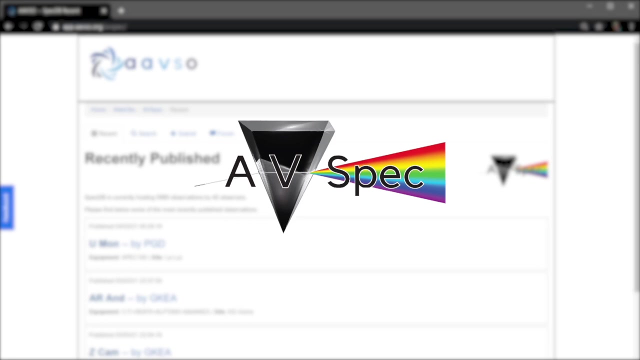 our own sun. And the best part, All of this fantastic data I collect with my telescopes can be submitted straight to AAVSPEC, the AAVSO's new spectroscopy database, where professional astronomers will be able to use my data to make new advancements in. 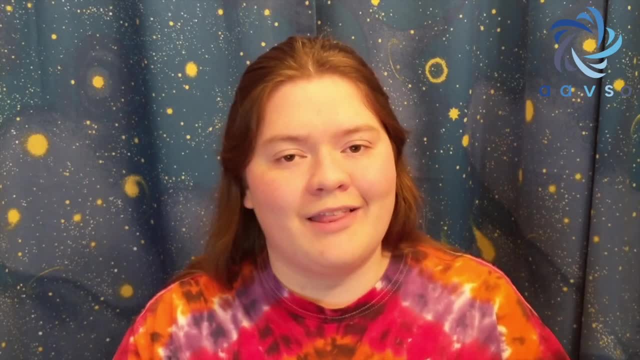 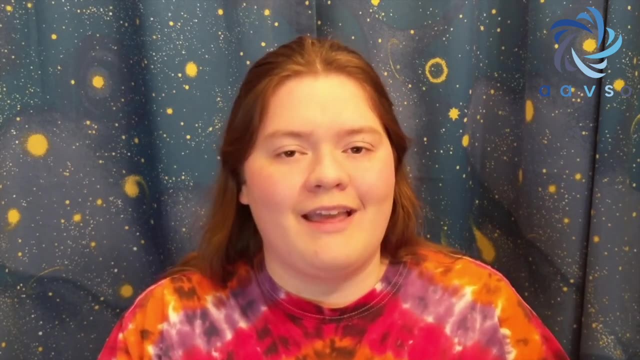 astronomical research. So are you interested? You can do this too. All you need to do to get started is join the AAVSO and request a mentor through our mentorship program. We will be happy to help guide you through every step of the way. 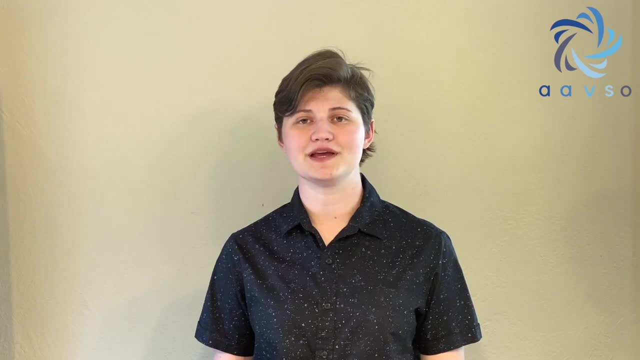 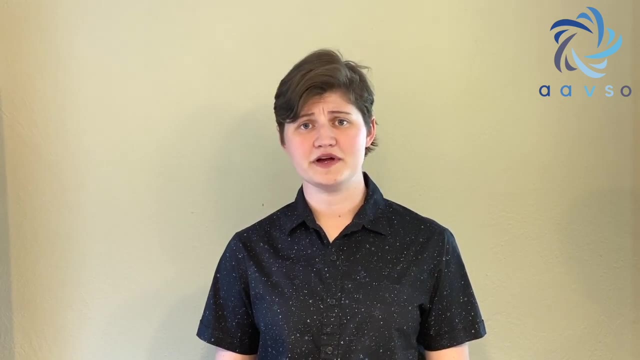 One of my favorite things about spectroscopy is how many different applications these measurements can be used in. Next we have Kelsey to talk about amateur astronomy organizations. They're an excellent way to learn about observance, but they're also an excellent way to learn about 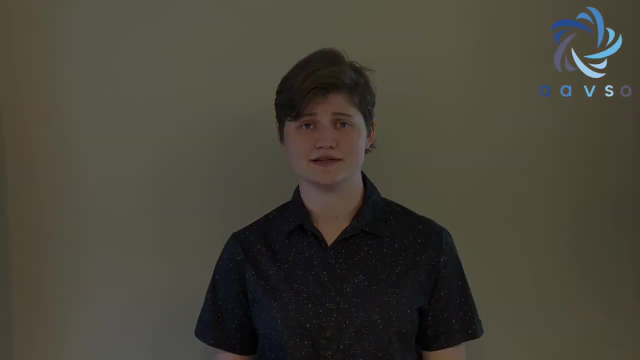 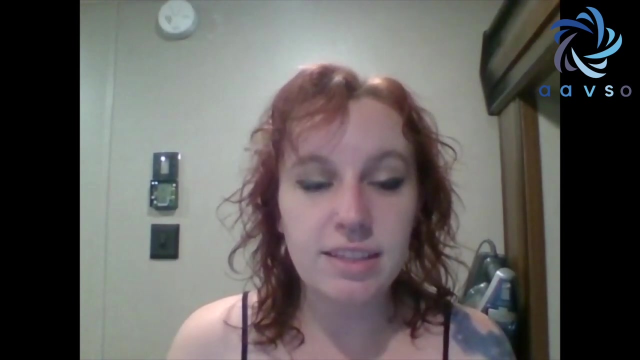 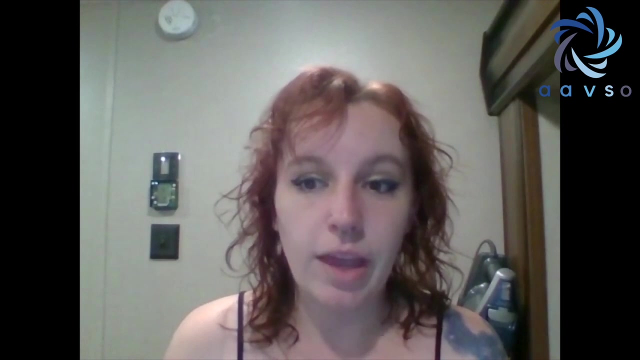 observing and offer many opportunities that will help you through this process. Hello, my name is Kelsey Davis and I'm from Southern California. My observing experience recently has consisted of a lot of work observing double star systems, and I do that as part of an outreach effort for my local amateur astronomy organization. 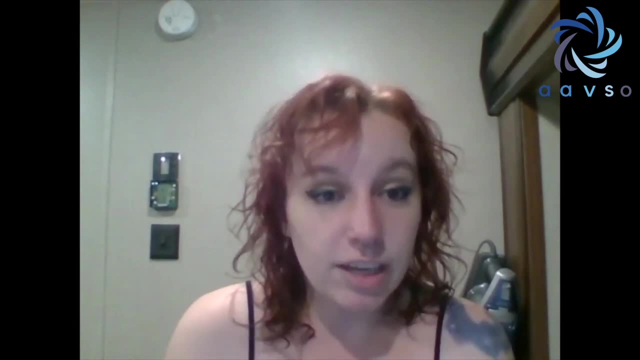 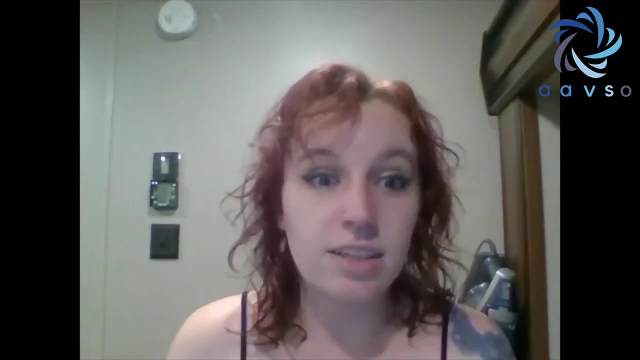 If you're new to observing, if you've been here a while, if you're looking to make connections, I would highly recommend that you look for your local amateur astronomy organizations. You'd be surprised. they're all around the country. That's where I've gotten a lot of 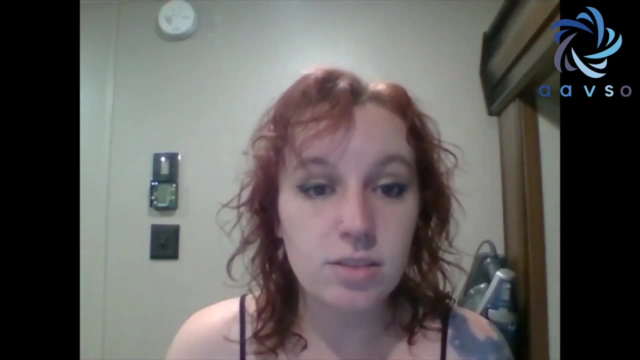 connections. Often it's a good place to look. if, wherever you are in your path, in observing whether you're brand new or whether you've been around a while and you're looking for new and interesting things to do, I highly recommend that you try to find your local amateur. 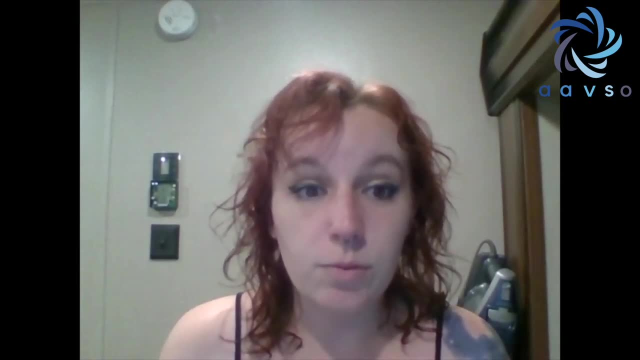 astronomy organizations. They also vary a lot, but they're all very similar in that they're all very different, So I think it's a great place to find your local amateur astronomy organizations. Very often we'll rent out telescopes, which can be a huge help if you're new to observing and. 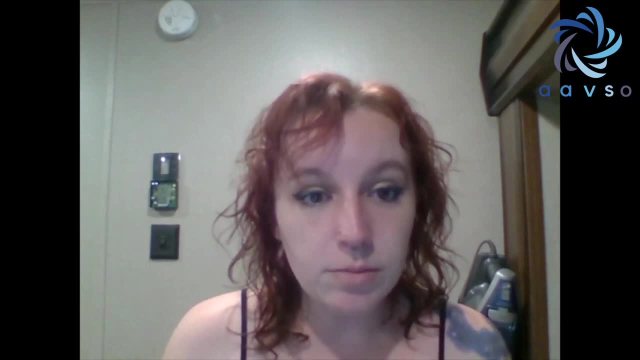 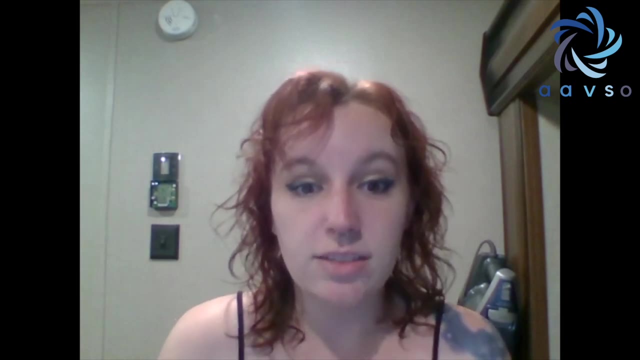 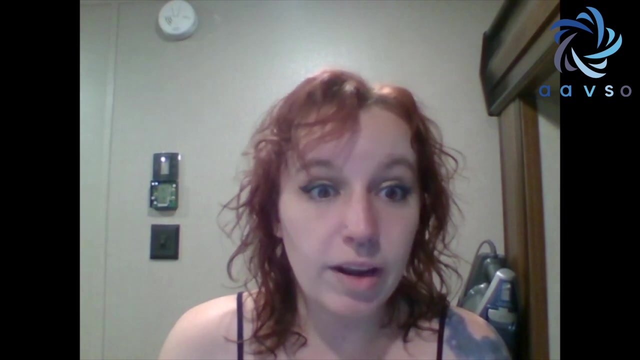 you need some help because telescopes can get expensive. I highly recommend that you take some time to search out your local amateur astronomy organizations. They're also a great place to not just bounce ideas off of other people that like to do observations, but it can be a great place. 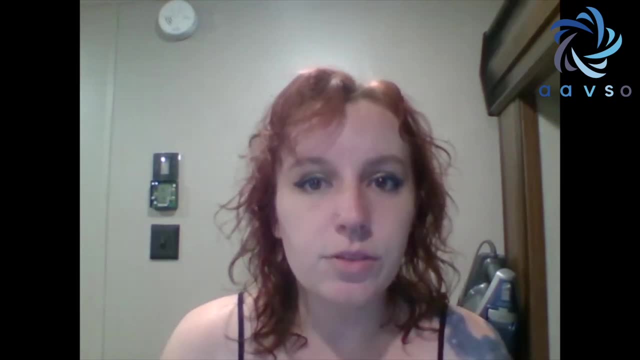 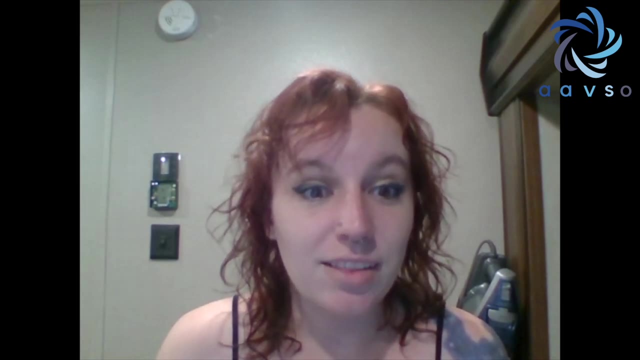 to take place in star parties. There's all kinds of cool stuff you can do if you get involved with your local amateur astronomy organizations. So I highly recommend that you take some time, if you haven't already, to find those people, because I'm sure there's people that would love. 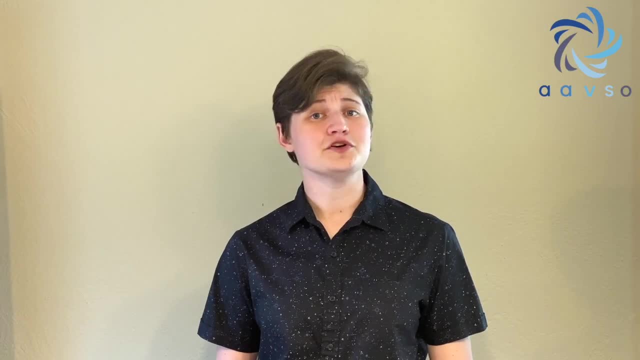 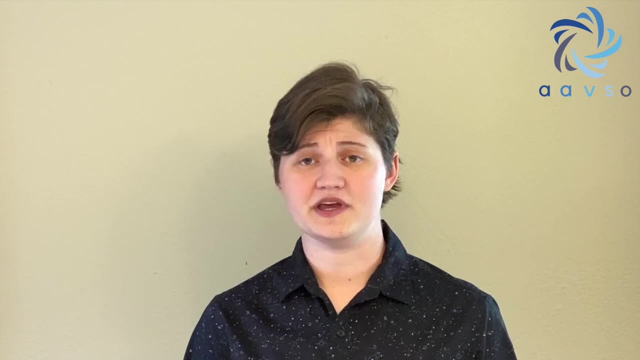 to work with you. If you have an organization near you, joining up with them would be a wonderful way to learn more about observing. Finally, we have Molly to talk about introductory astronomy equipment. Hi, my name is Molly Wakeling and I'm an ambassador for the American Association. 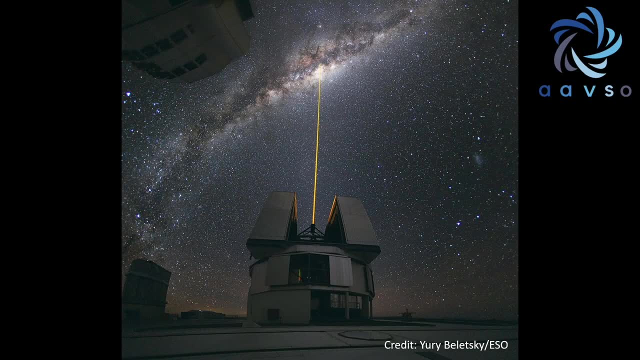 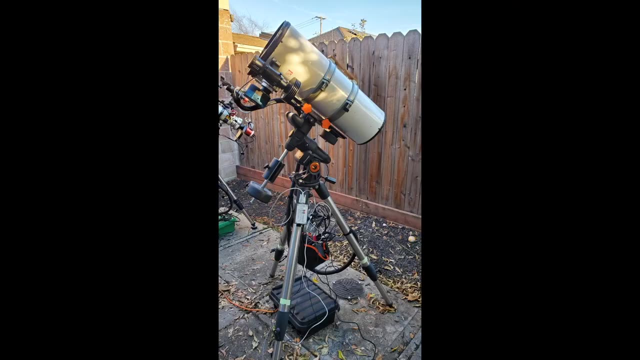 of Variable Star Observers. You might think you need some big fancy observatory to do variable star measurements, but oftentimes you can use equipment you already have. This is my rig: an old 8-inch F4 Newtonian that was passed on from another amateur astronomer, a QSI 583 CCD camera. 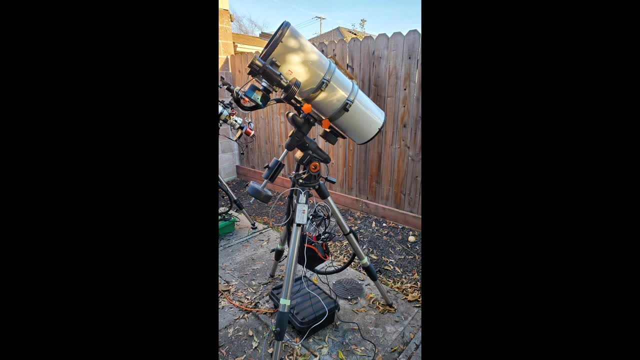 and a Celestron AVX mount. Admittedly, the QSI 583 is a relatively expensive camera, but I happen to have one. You can use a wide variety of CCD or even CMOS cameras. You also don't have to live under dark skies. I image from my backyard here in the San Francisco. 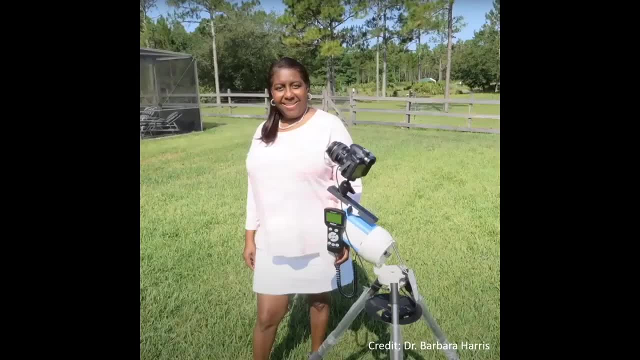 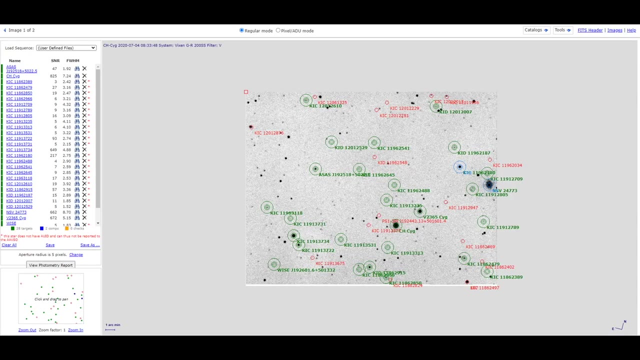 Bay Area. You don't even need this fancy of a rig. AAVSO observer, Dr Barbara Harris, measures variable stars using a DSLR and a camera lens. There is even a tutorial document on the AAVSO website on how to do DSLR observing. You also don't need fancy software. I happen to already. 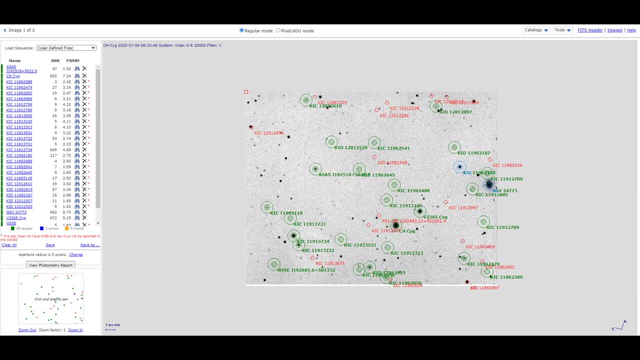 have PixInsight, but you can use a variety of image processing software to do the pre-processing, such as the free DeepSkyStacker, since you just need to calibrate and register your images before uploading to the VFOT online software provided by the AAVSO for analysis. So come be a part of. 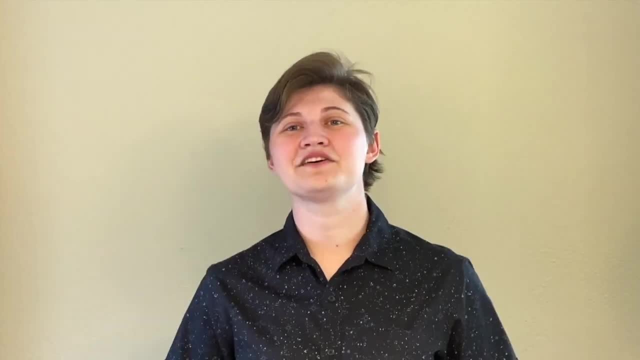 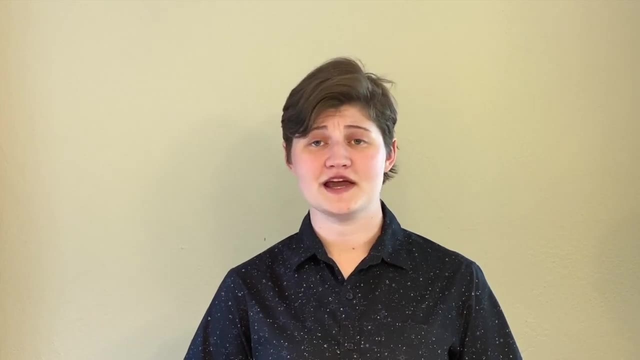 astronomical research with the AAVSO. And that concludes our video for the day. I hope you all enjoyed and maybe even learned something. There are a lot of resources offered online at our website, AAVSOorg. Thank you for watching and I'll see you next time.